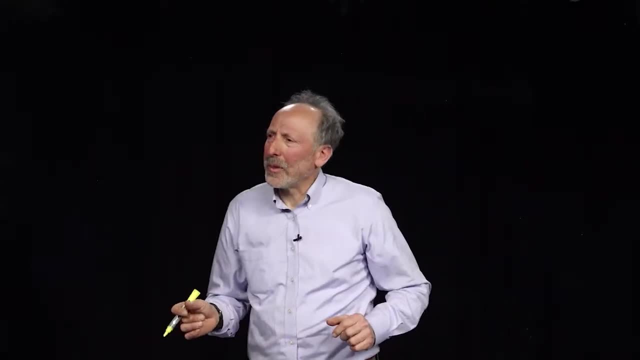 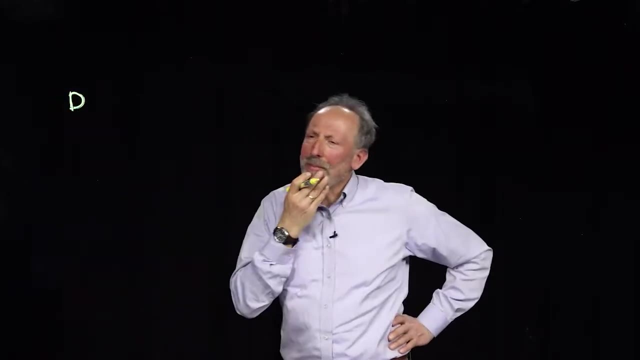 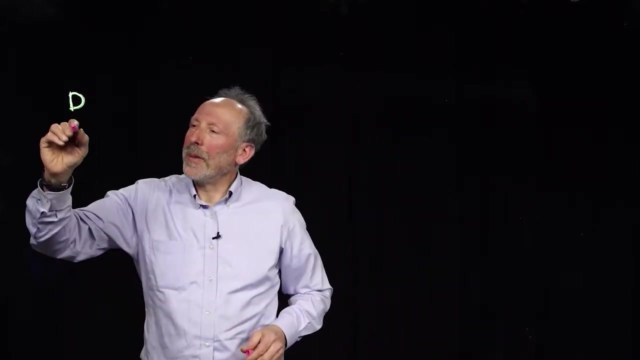 When we've talked about dispersion of plumes, we've used a, D and we've said, okay, that's the dispersion that we're going to use in our differential equations. But there are two processes which give rise to dispersion. One of them is diffusion and one of them 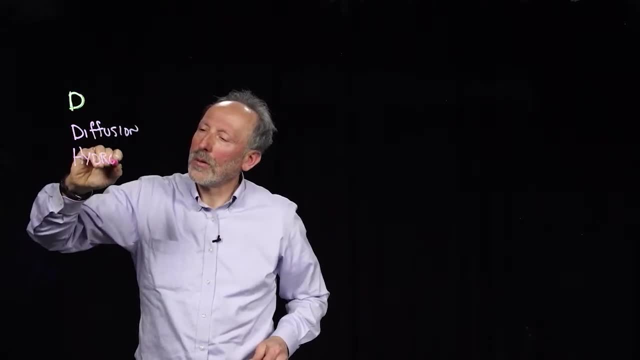 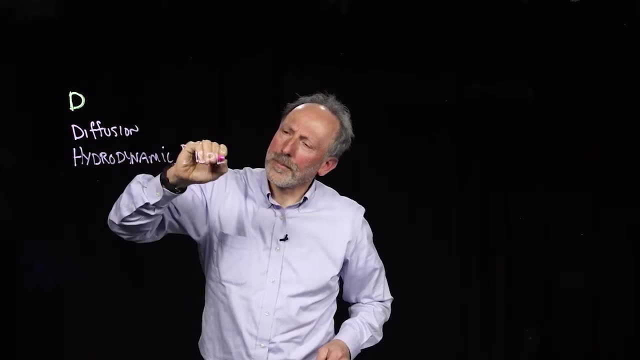 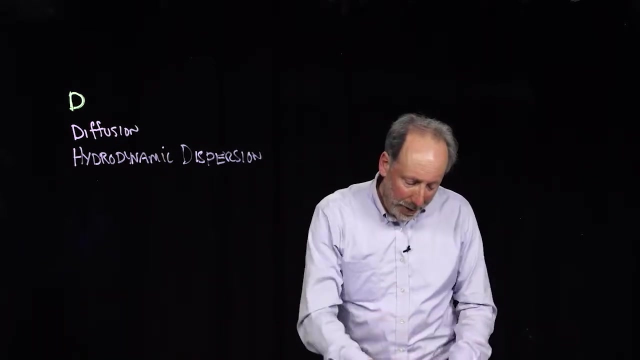 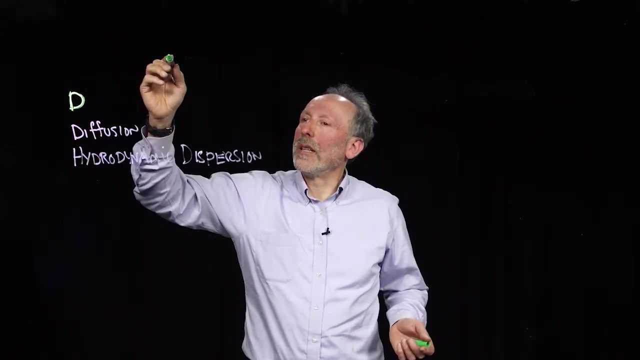 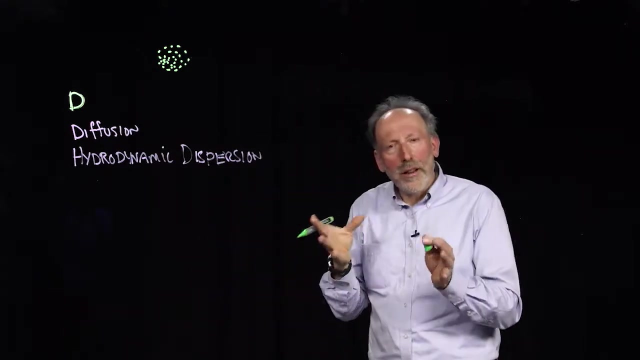 is hydrodynamic dispersion. Okay, So we have these two things. So when we talk about the classical diffusion- and this is something that actually Einstein was really material in developing understanding- you basically have a set of molecules in space And they all have energy and they're all vibrating And so, in time, this plume of 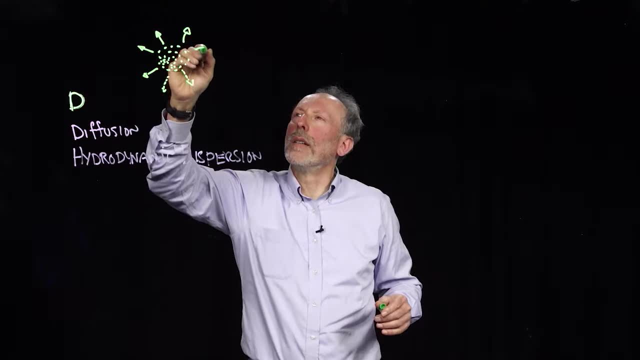 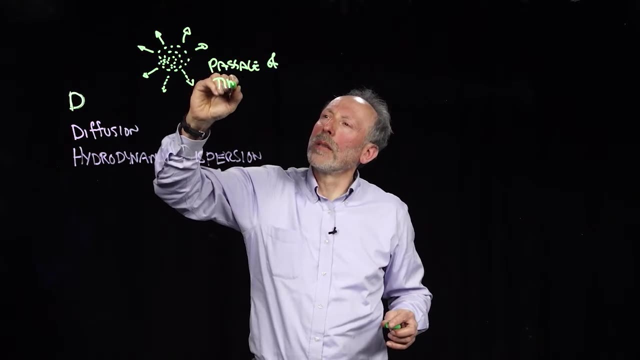 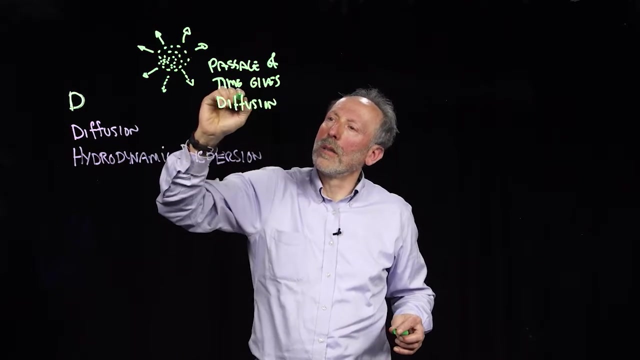 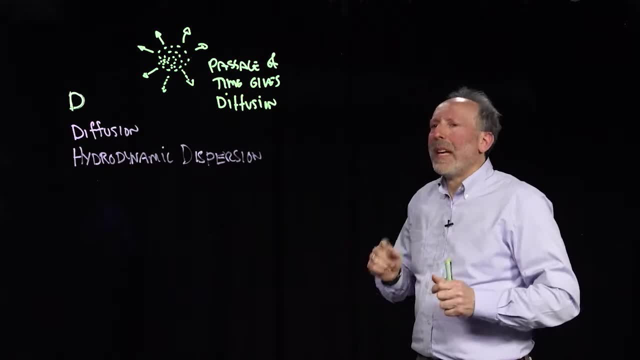 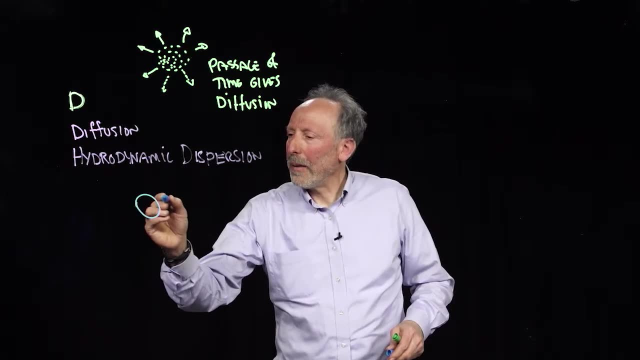 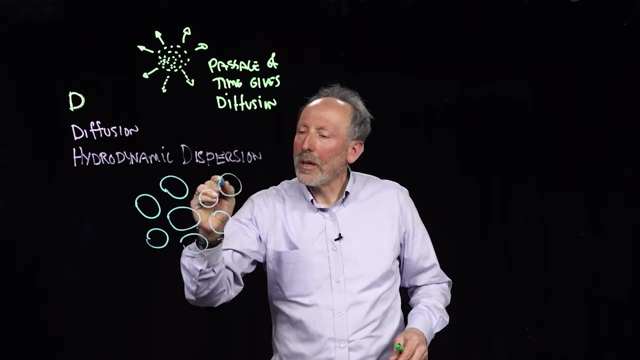 very subtle time, But it will happen. whenever time passes, Things will diffuse. Dispersion, on the other hand, is very different. Dispersion is when we have a media, let's say, and we're going to push our solute through that medium. 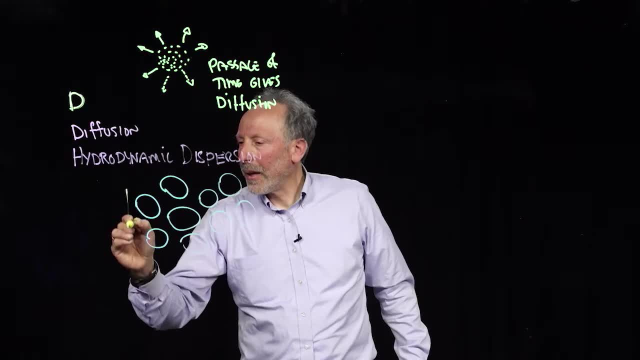 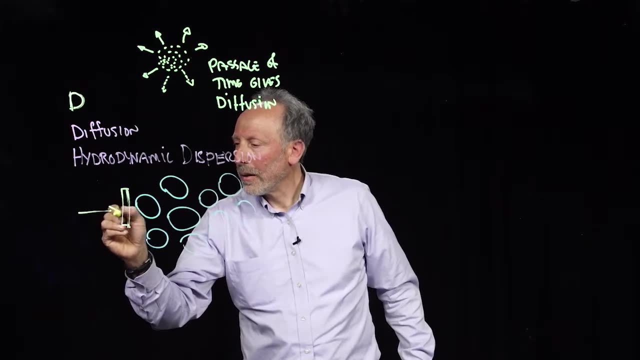 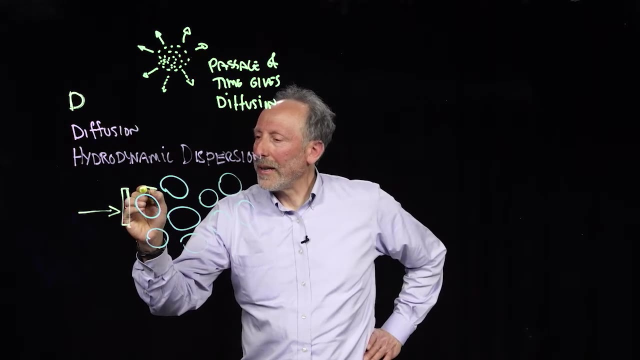 And so what's going to happen is that if we start with solute in this form, as the water flow pushes the solute through, then this is going to deform, And so we're going to end up with at time two- this is going to be at time equals zero. 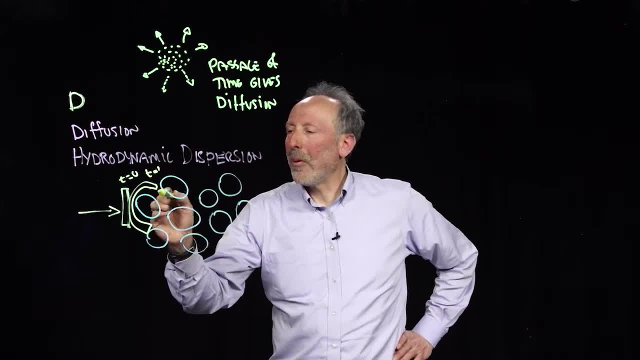 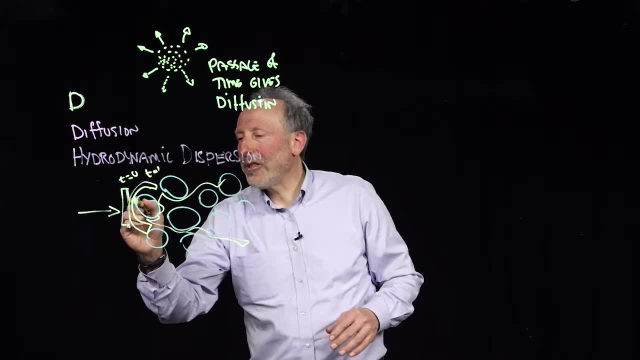 at time equals one. it's starting to bend and then at some point this is going to be deforming all throughout this system, as it has stagnation points and high velocity points. so the plume is actually getting sheared apart. 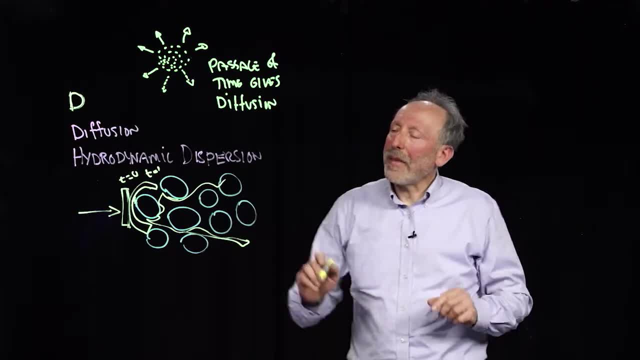 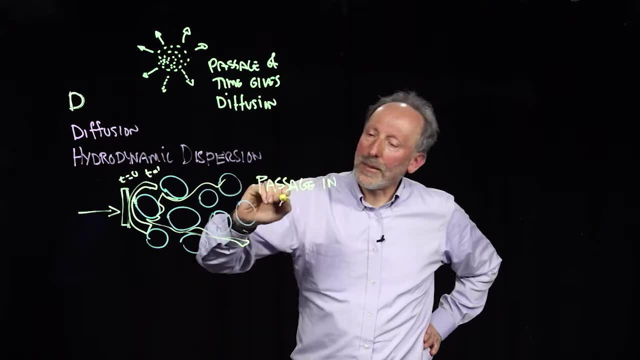 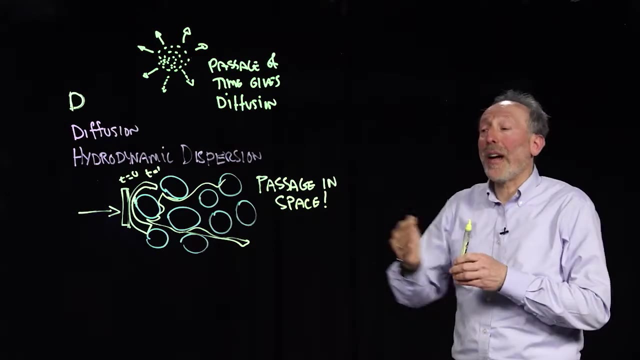 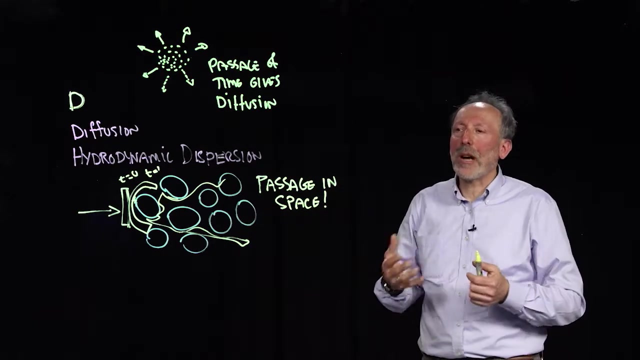 And that's hydrodynamic dispersion. So what do we see that's different about this? This occurs with a passage in space, So hydrodynamic dispersion is a function of how far something's been displaced, not how long it's been there. So there's two fundamentally different processes which we wrap up. 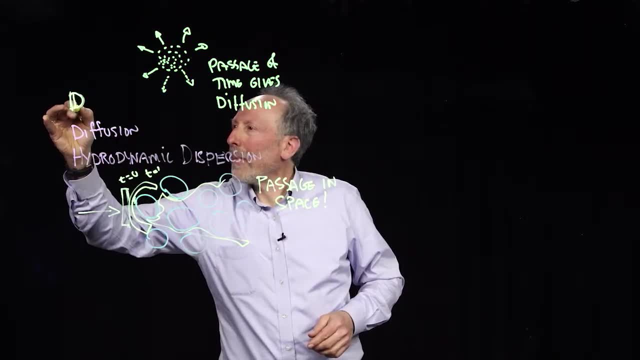 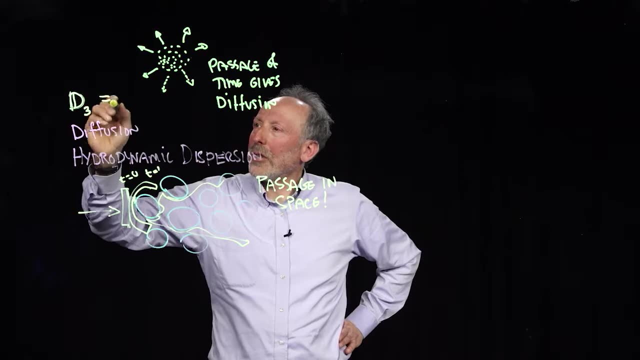 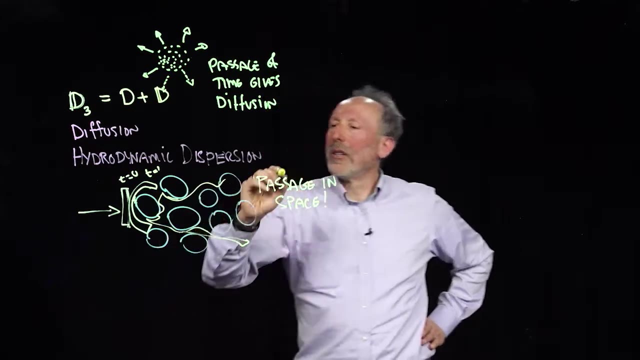 In a single D and I'll often write it as a double back with a three there, and that I will call the joint hydrodynamic dispersion, which is going to be a function of diffusion plus dispersion. So I will call dispersion a double back D and I'll put the three under it and call that. 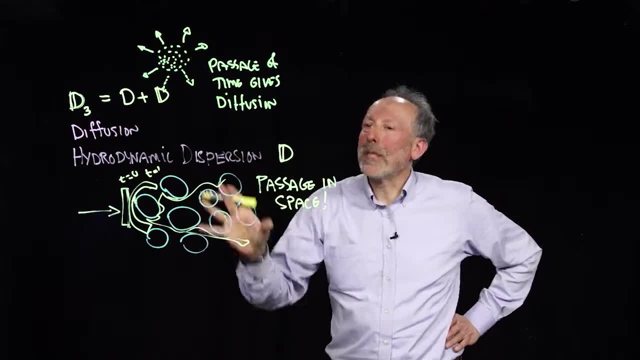 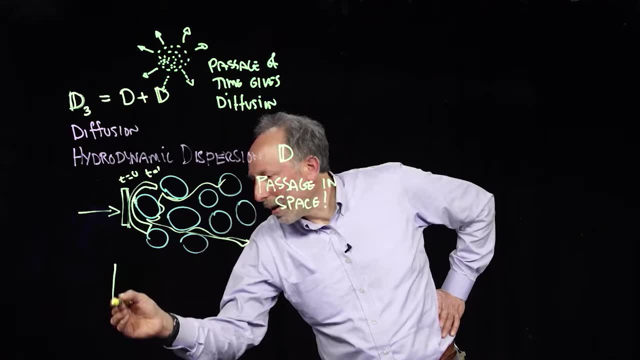 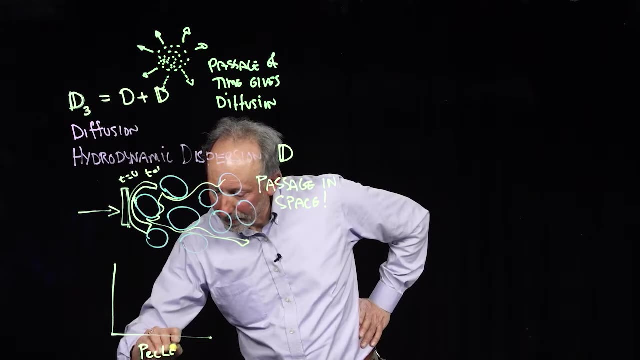 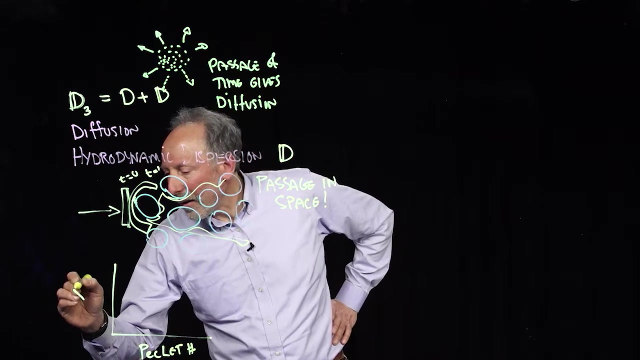 the sum of the two, And so that would be the types of dispersion and diffusion that we have, And what we do then. What we do then is we draw what's called, We calculate the Peclet number, And what it is plotting is the effective hydrodynamic dispersion over the diffusion. 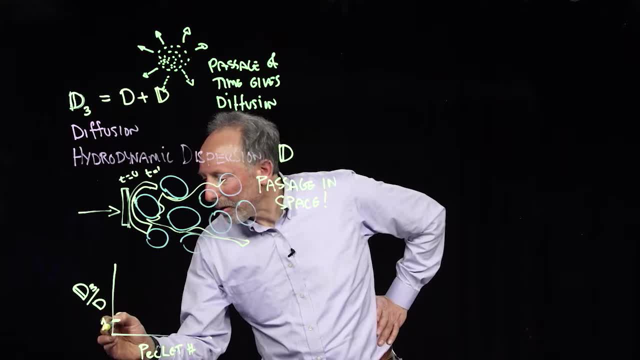 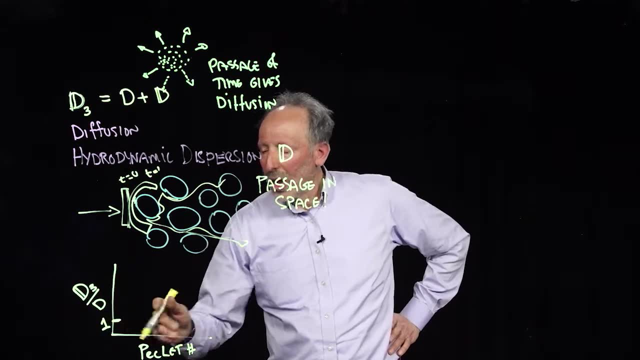 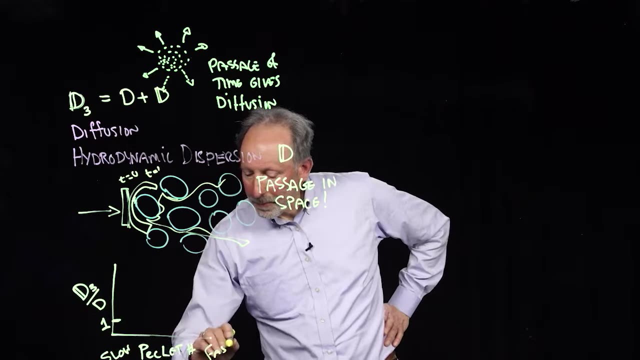 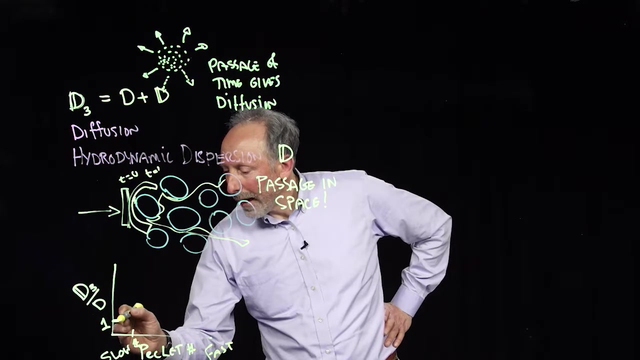 So at low Peclet number, this has a value of one, which means that this is equal to that. So it's diffusion dominated. So when things are going slowly versus fast, and then as we cross a Peclet number of one. 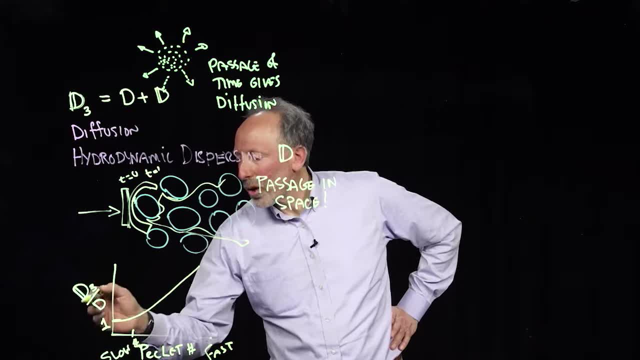 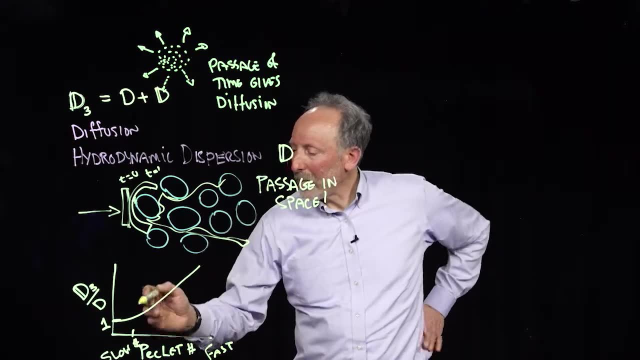 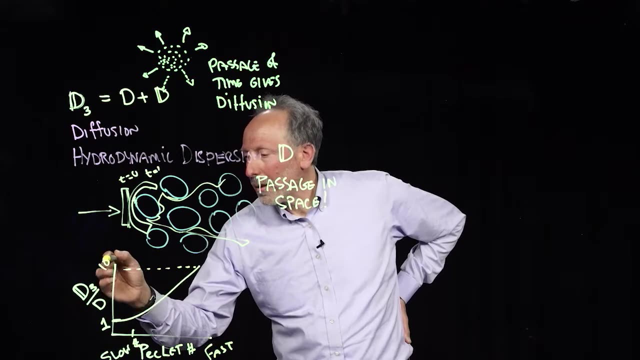 then this curve bends up and we get more and more contribution to the spreading process due to the hydrodynamic processes. So a typical, When we A typical Peclet number curve will look like this: This can certainly get into values of, you know, hundreds times greater than diffusion. 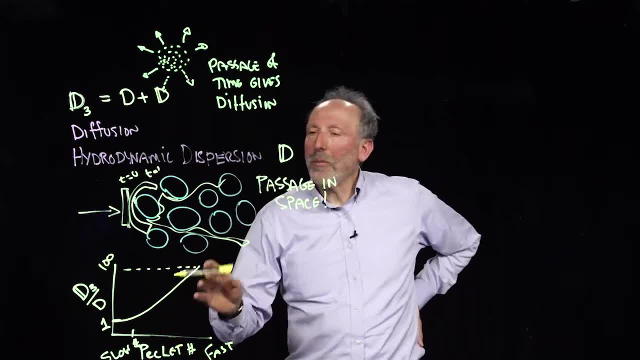 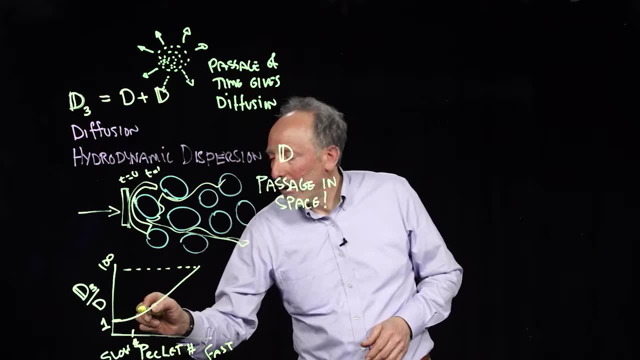 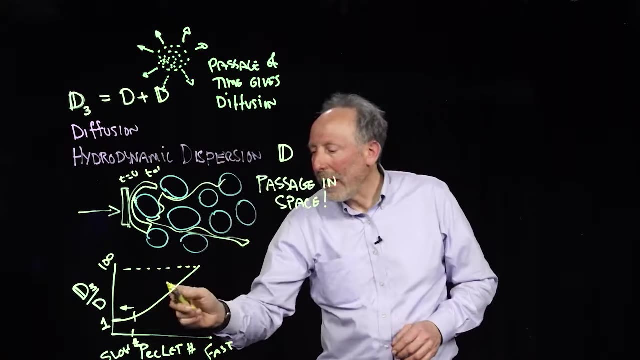